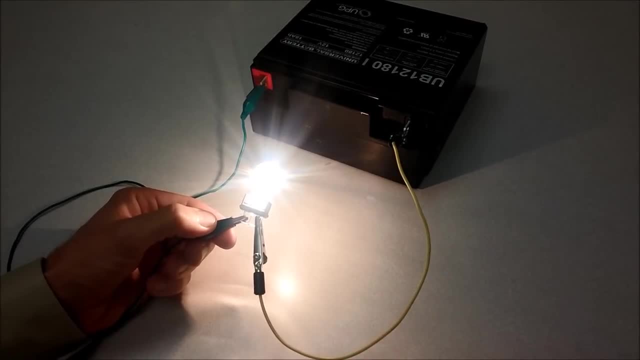 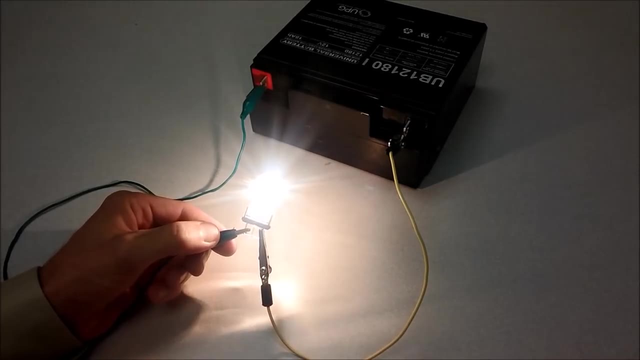 and bring it over here and it would stick to the wire, but it doesn't. But that doesn't mean that there isn't electromagnetism. It just means that the magnetic field isn't very strong around a single wire with a small amount of current flowing through it like this. So 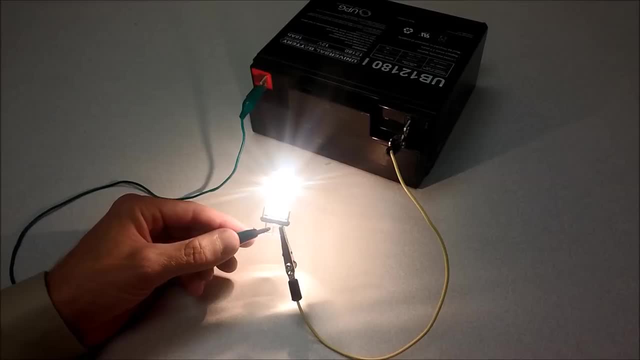 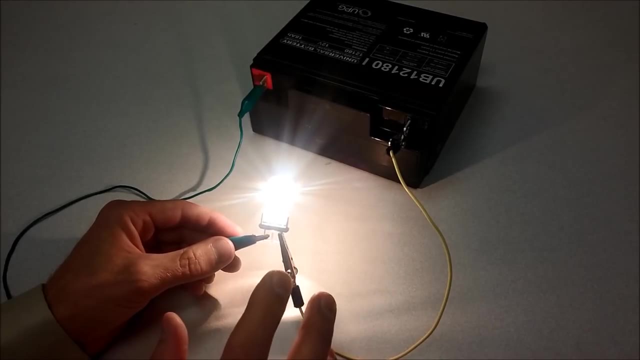 we're going to connect the wires to the battery and connect them to the light bulb For electromagnetism. what we end up doing is creating a coil where we wind the wire around an iron core several times And by doing that we concentrate the magnetic field and it's strong. 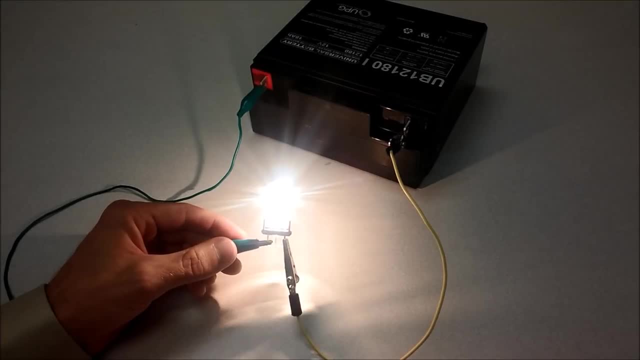 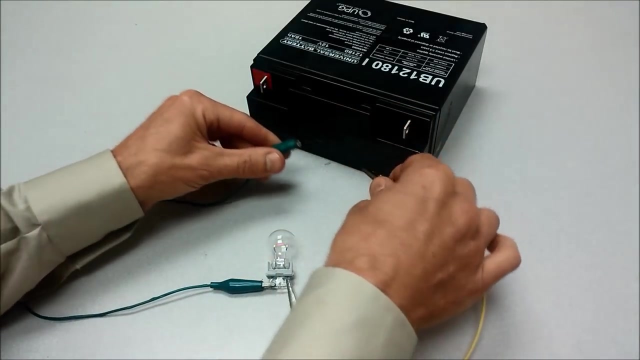 enough that this would happen, And I'll show you in just a minute how that works. The second principle is the principle of induction, And that says that when a magnetic field passes over a wire, it will induce or create electricity and electrical current in the wire. So according to that theory, 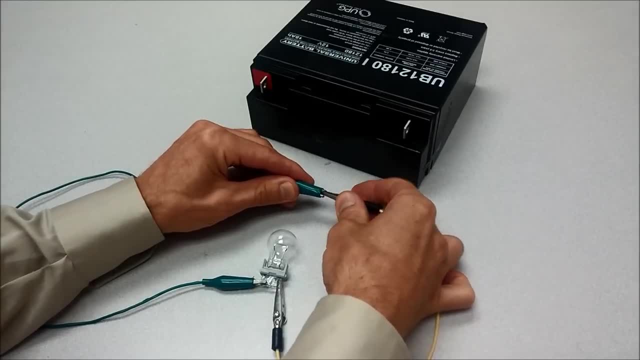 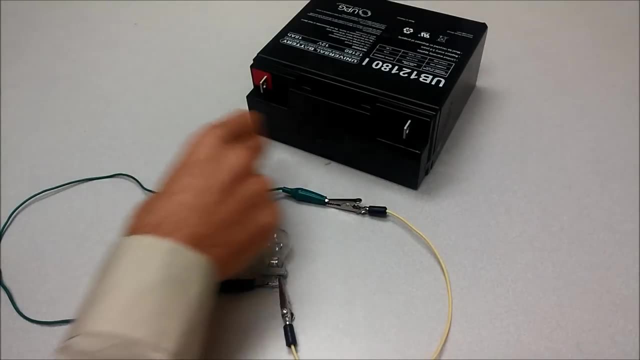 we can create a coil where we wind a wire around an iron core several times And by doing that we think we can probably eliminate the battery. Just bring the wires over here like this: Let's grab our permanent magnet and come over here and move this across the wire and we would hope to see the 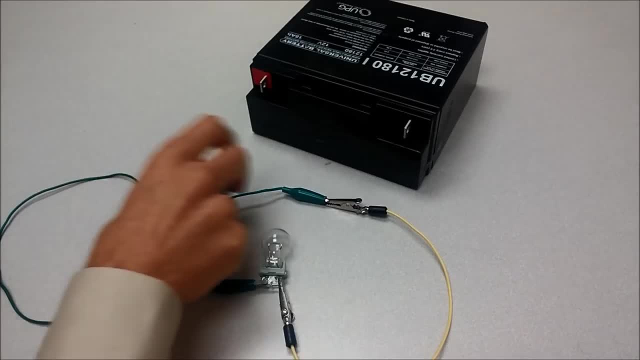 light bulb light. Again, it's obvious that it doesn't work, But that doesn't mean that we're not creating electricity. In order to use this principle, to create enough electricity to light that light bulb, we would need to create a coil, So we would wrap the wire around an iron core. 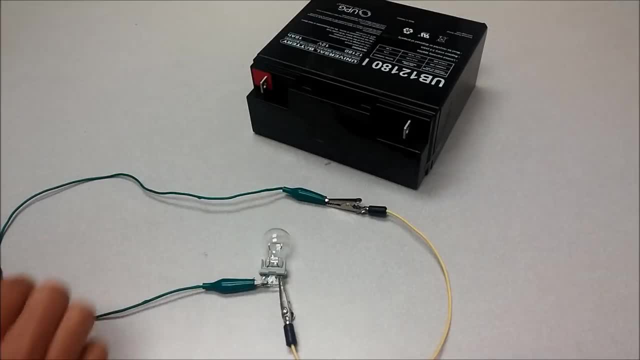 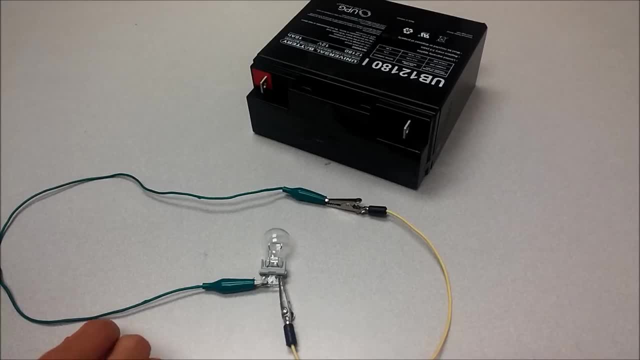 light, a light bulb, or power some other device. Now I should mention, when it comes to induction, that the magnet or the wire needs to be moving. We can't just set a magnet on the wire and expect that magnetism to create any kind of a current. It's actually the magnet passing over the wire. 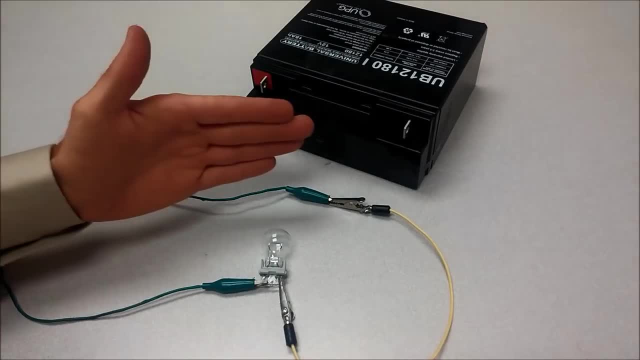 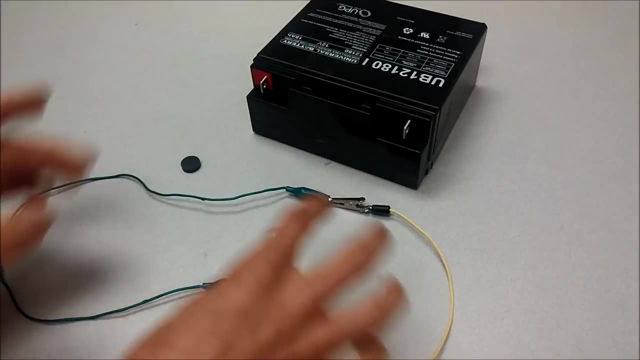 which causes the electrons to dislodge and to be pushed in the circuit. So when I do this, when I move this magnet back and forth, there's literally a push and a pull of electrons moving in the circuit. It's just that it's so small. in this case it doesn't light the light bulb. That's the. 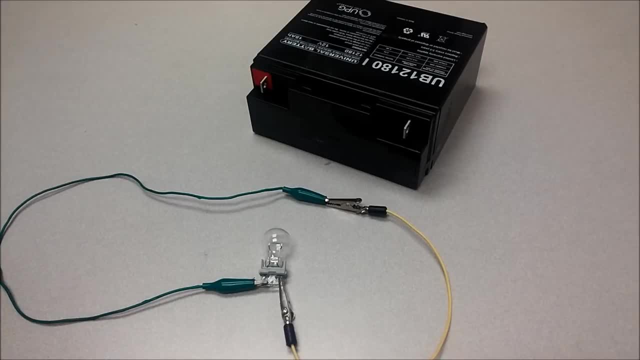 principle of induction. So, basically to summarize, when electricity passes through a wire, there's a magnetic field that is generated around that wire. So electricity makes magnetism. On the flip side, when a magnet passes over a wire, electricity is created in the wire. When a magnet passes over a wire, 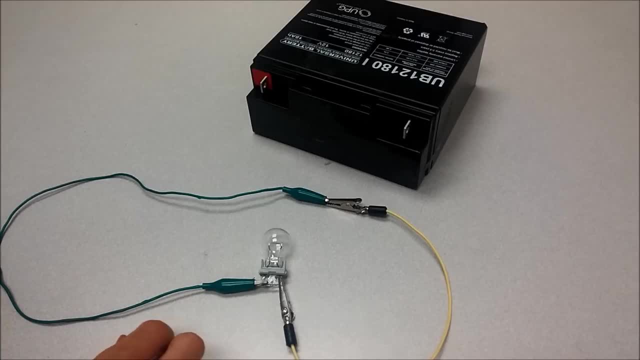 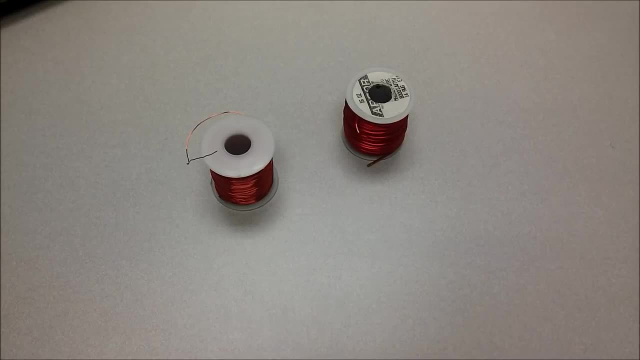 electricity is created in the wire. When a magnet passes over a wire, electricity is created in the wire, So magnetism creates electricity. It goes both ways. Okay, over here I've got a couple of rolls of magnet wire and it's just really wire At first. 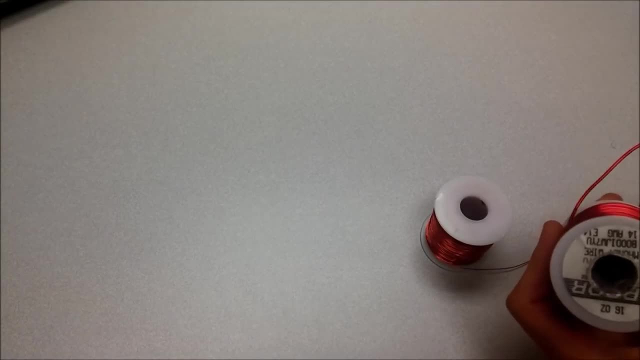 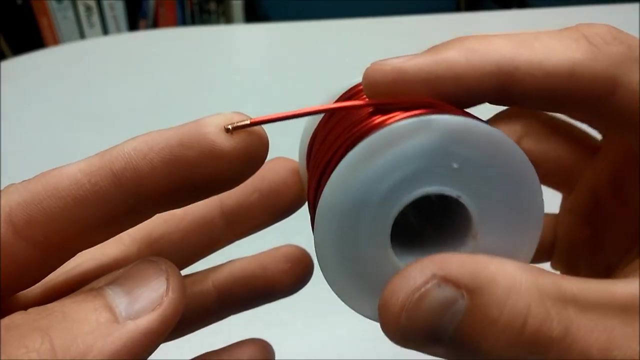 glance you might think there's no insulation on this, but it does. This red coating is the insulation. You'll be able to see where I've stripped off that coating. You can see the copper center. It's a solid core wire. It's got a copper center with an insulating coating. 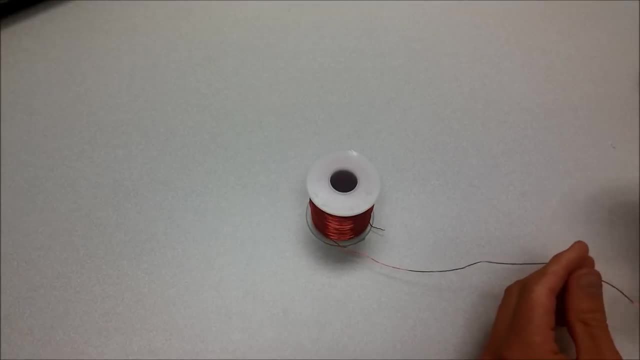 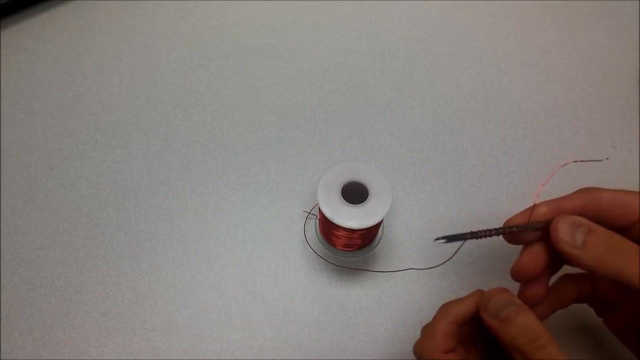 over top of it. Now what you could do with this is take a nail or a screw or a bolt or something and take some of this magnet wire and just wrap it around many times As you do that. we've created a coil Now when we apply voltage to both ends of this wire. so if I was to cut this off and 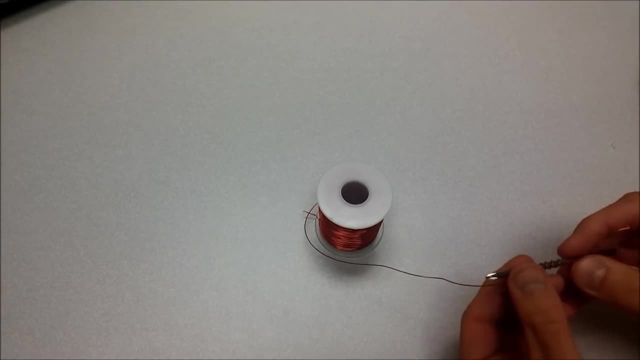 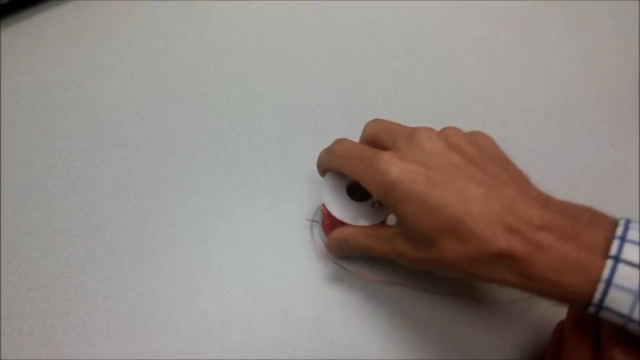 connect each end of this wire to a battery, we will have concentrated the magnetic field enough that whenever there's current flowing through this wire, the current will flow through the wire. It'll become an electromagnet. Now just to show you an example of this: 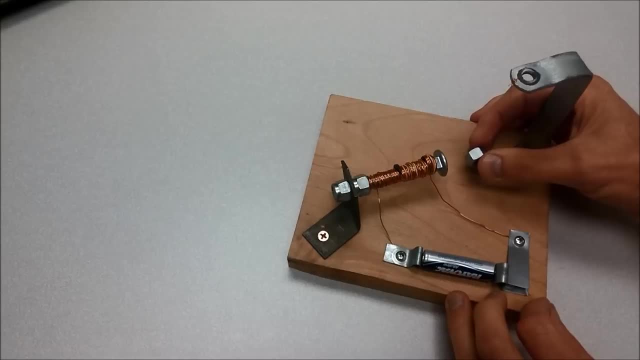 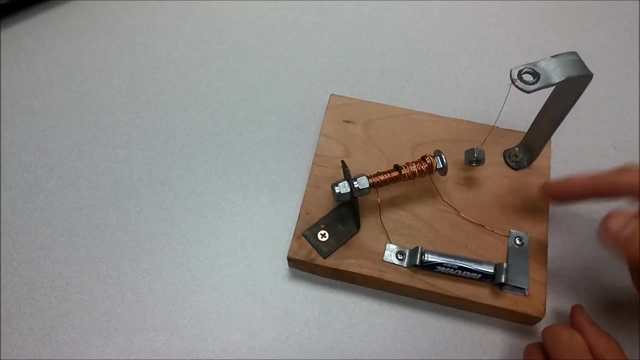 I've got this little device here, A little homemade device. All this is, if you look at it, it's just a bolt and it's just connected to this bracket that holds it up. so it's a bolt and it's got a piece of magnet wire that's been wrapped around it. It looks like maybe. 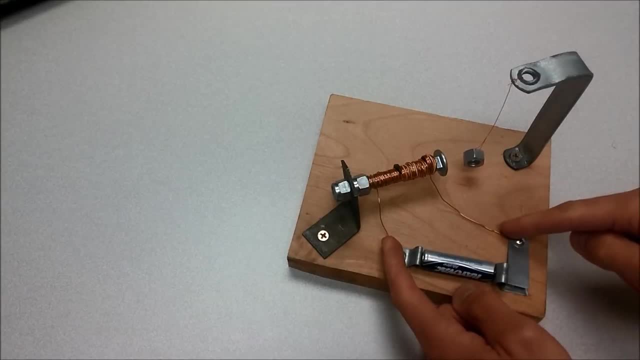 50 or 60 or 100 times. And here are the two ends and they connect to this battery. I've just got a little switch here, so when you connect this, when I want to connect this you're I push this button. you'll watch. this nut that's hanging from this wire is pulled. 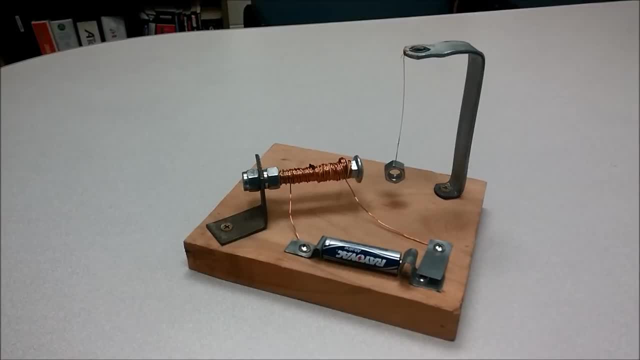 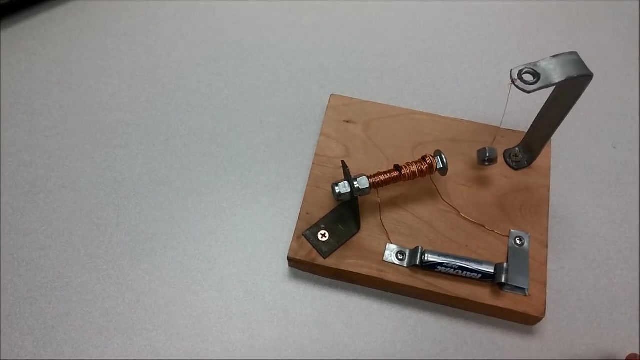 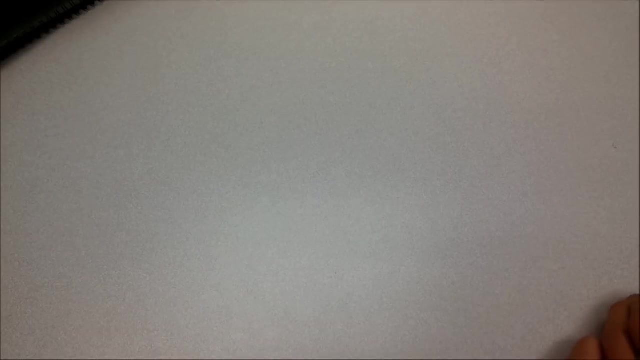 over immediately, and when I let go it, it releases it. so that's the principle of electromagnetism. use that in relays. we use that in a lot of devices: electric motors, solenoids. here's a great example of how electromagnetism can work. this is. 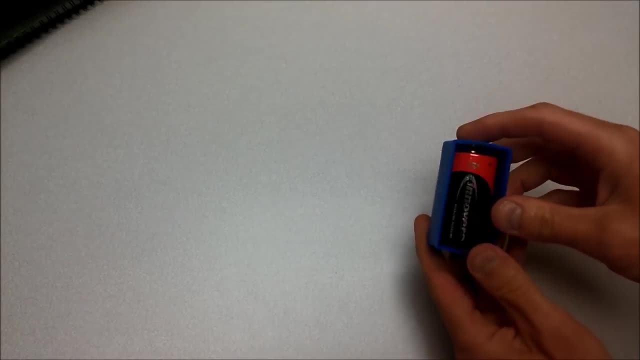 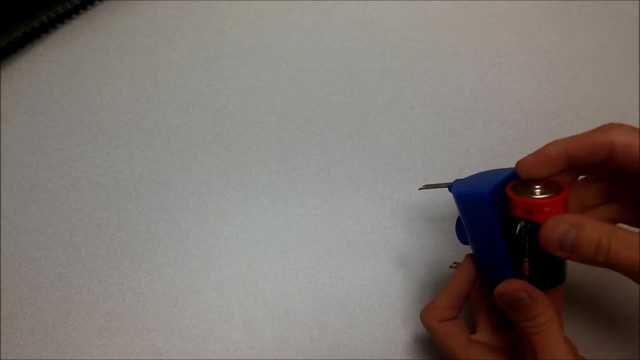 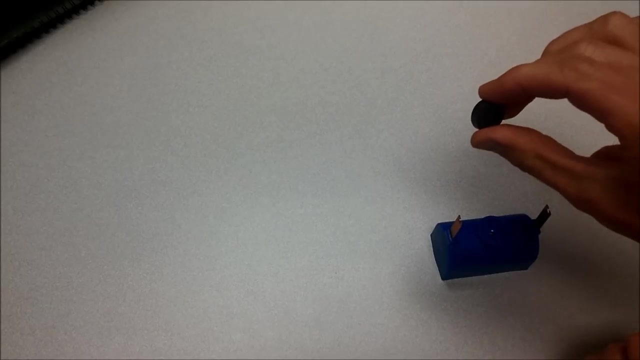 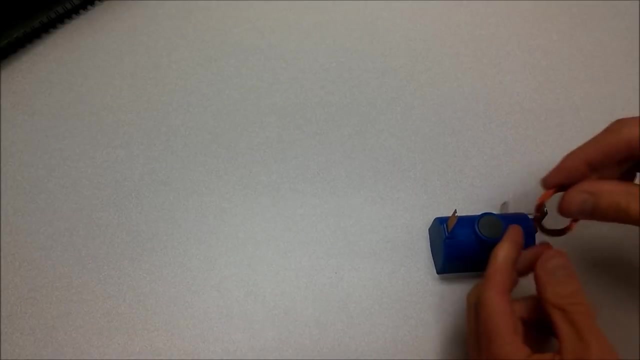 just a simple battery, and this battery connects to these two terminals, so I place it in here. these two copper terminals are touching the battery. then we have a permanent magnet. so this is the type of magnet you'd find on your refrigerator. it's a permanent magnet that drops down into that hole and right here we've just taken a piece of this. 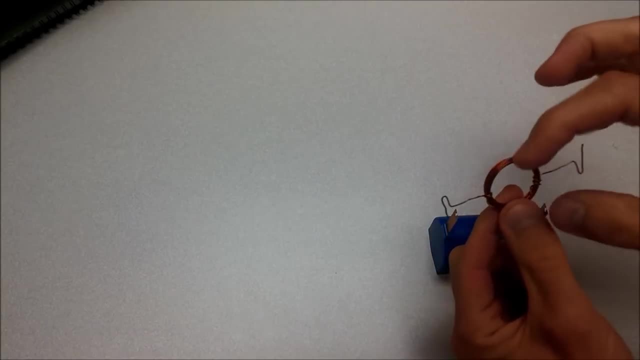 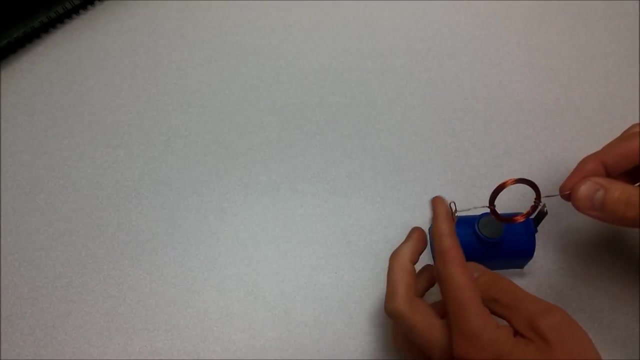 magnet wire, wrap it around a cylinder just to make a loop, and I've got both of the ends right here. so if you look at it, it's just been wrapped around now. when we set that in here, I scraped some of that coating off of the copper wire, so 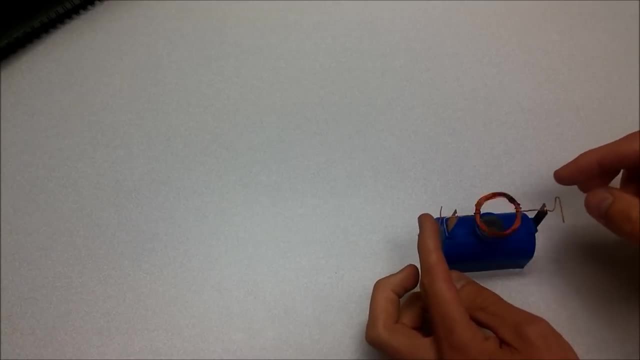 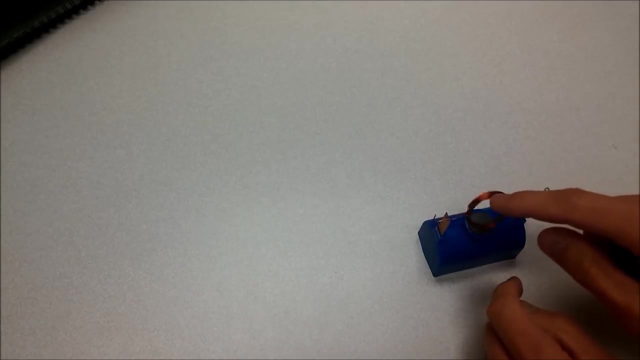 that it can touch these contacts. you'll see there immediately you can sell. something's going on. it's creating a magnetic field around this loop right here. that's either repelling or attracting magnetic field of this permanent magnet. so we get it just right. we might get to work it. it'll spin like a motor, but it's it's a. 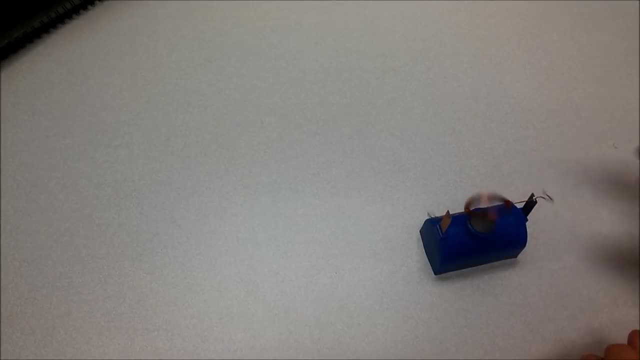 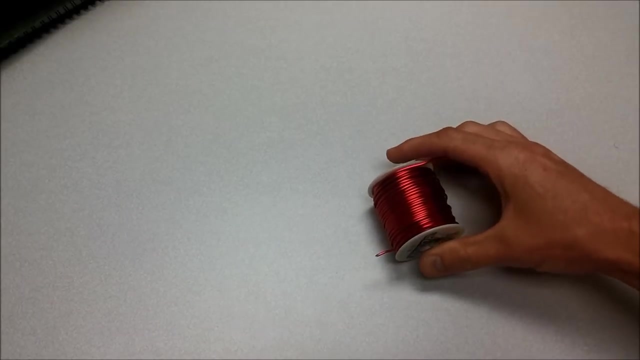 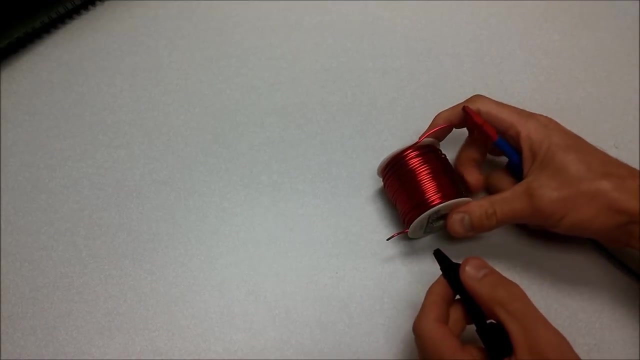 great example of how we use electromagnetism. now I'm going to show you how induction works. so I'll bring over one of these spools of magnet wire again, and because I'm going to induce a very small current, small voltage, I am going to be using the lab scope so that 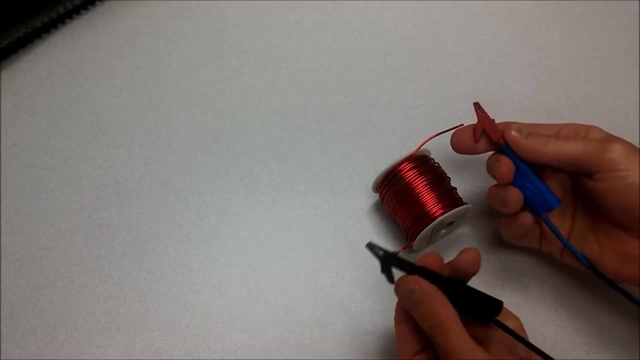 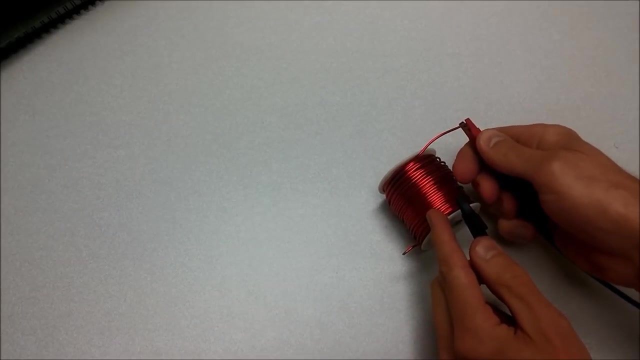 we can see this. I've got my leads to my lab scope. The lab scope is set on voltage and I'm just going to connect this on to the ends of these wires where the coating has been stripped off. So this is one single wire. this is just both ends. 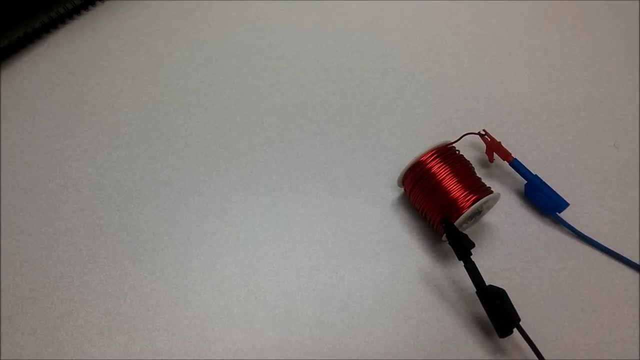 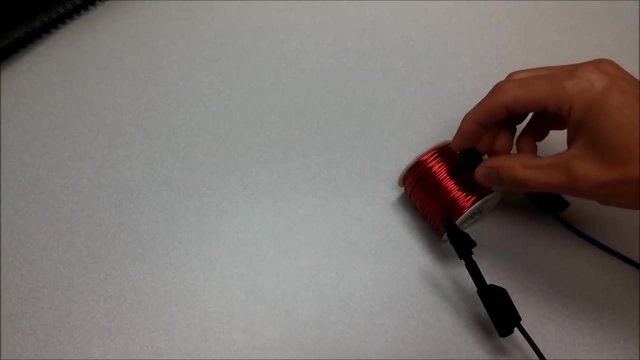 of the wire, And so I'm going to grab our permanent magnet that we just saw a minute ago and I'm going to come over here and remember that I can't just place the magnet near the wire and hope for something to happen, so I've got to move it. 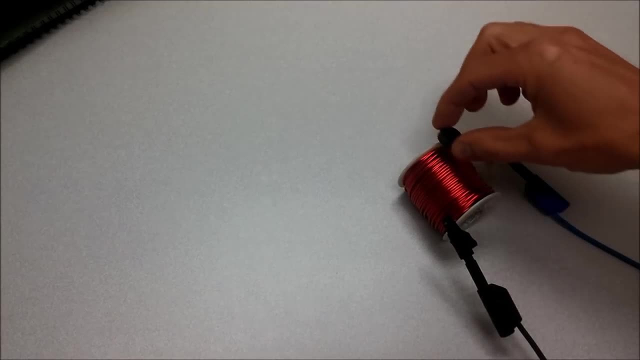 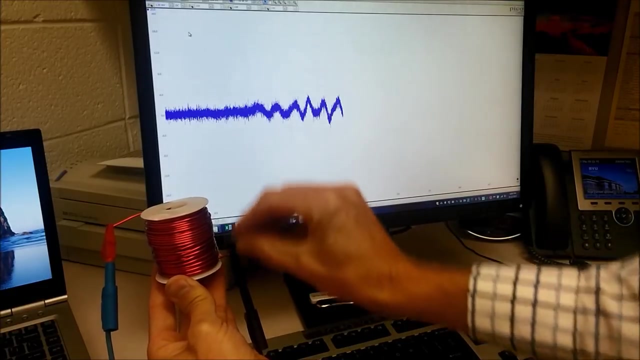 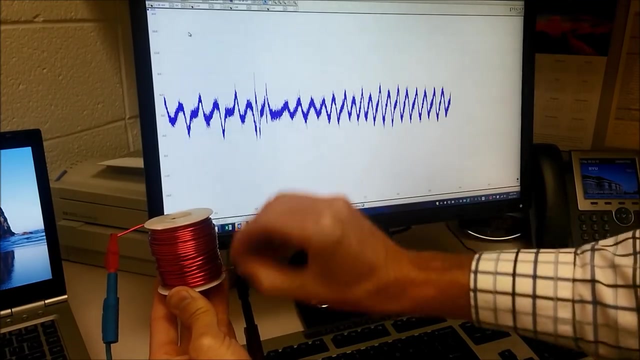 I'm going to come over here and move this back and forth across this wire And as I do this, it's generating electricity. You can watch as the electricity is generated. you'll see the voltage going up and down. The faster I go, the faster it goes up.